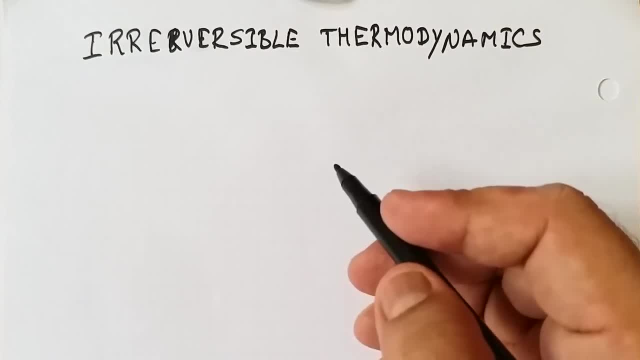 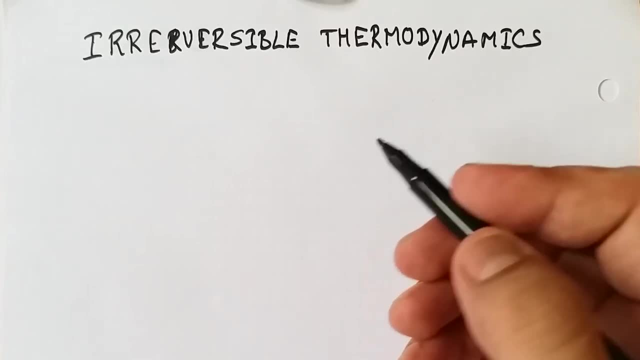 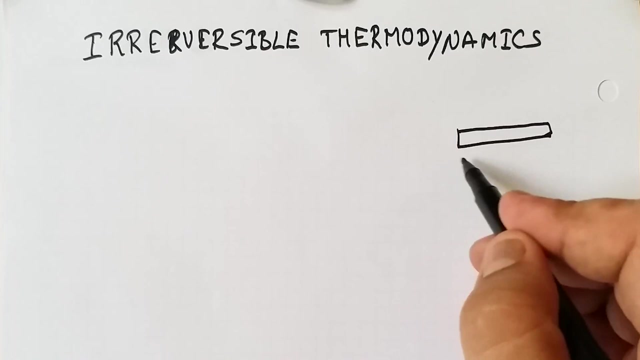 So there are several transport phenomenons which are irreversible. So these phenomenons, like we may say that there are a few examples. The first is the transport phenomenon, which includes the flow of heat along a metal rod which are kept at different times. So we have metal rods and we have T1 over here, T2 over here. So suppose this is a higher temperature and this is a lower temperature, then the temperature will flow from the end, with higher temperature towards the lower temperature. 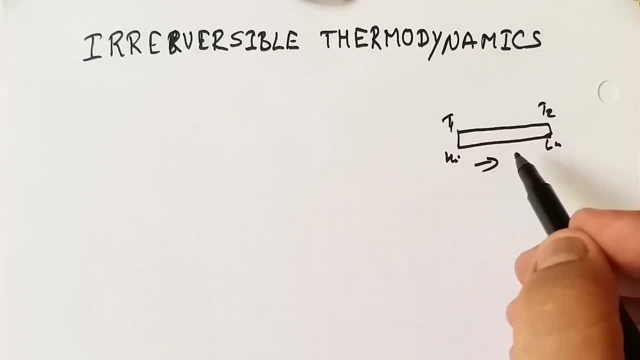 And this will be basically an irreversible process. So, similarly, the flow of the electrical current or the generation of heat, a development of heat when electric current flows- is also one of the example of irreversible process. Similarly, the diffusion of solids or, if we look at solids, or the diffusion of several fluids across the concentration. 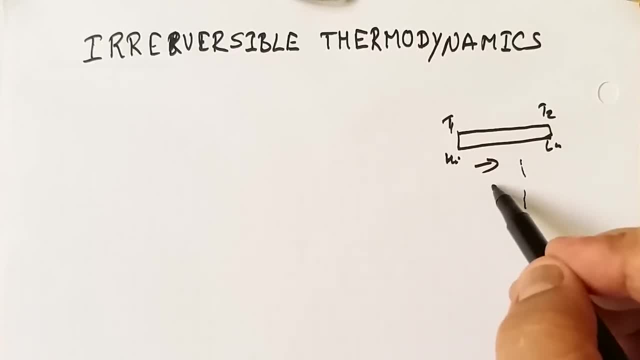 gradient. that is suppose, we have a semipermeable membrane and we have a concentration over here x and we have concentration y, then there will be flow through this semipermeable membrane, and that also too will be an irreversible process. so in short, irreversible processes they may be. 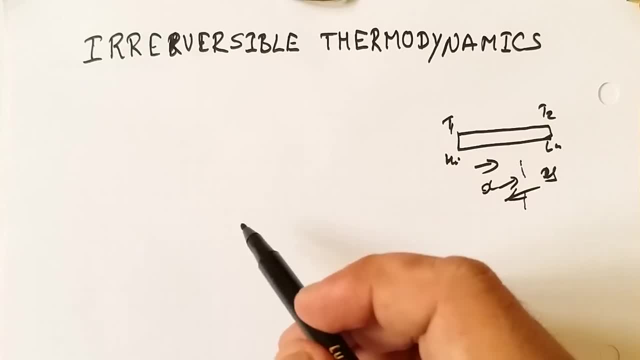 defined or irreversible thermodynamics, or it is also known as non-equilibrium thermodynamics. so this non-equilibrium thermodynamics, it can be defined as it is the branch of the science which is dealing with the study of thermodynamic properties of a system which are not in. 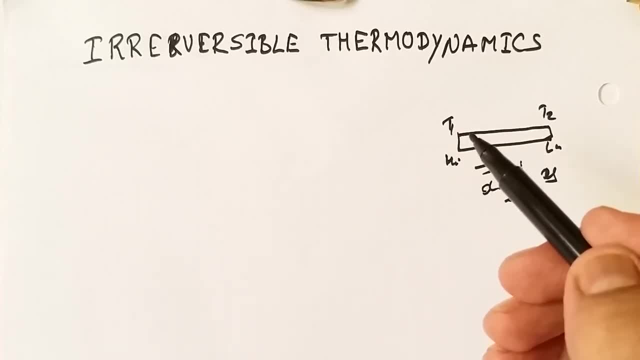 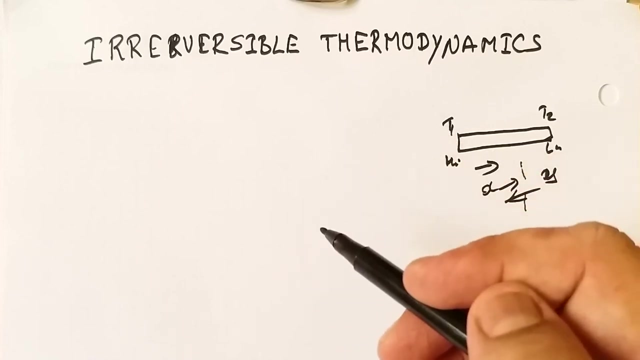 equilibrium and they involve transport processes which are irreversible. so this is termed as the non-equilibrium or irreversible thermodynamics, or it is also known as thermodynamics of irreversible process. so this is the typical textbook definition of irreversible thermodynamics. now, in order to develop this particular theory, there are some. 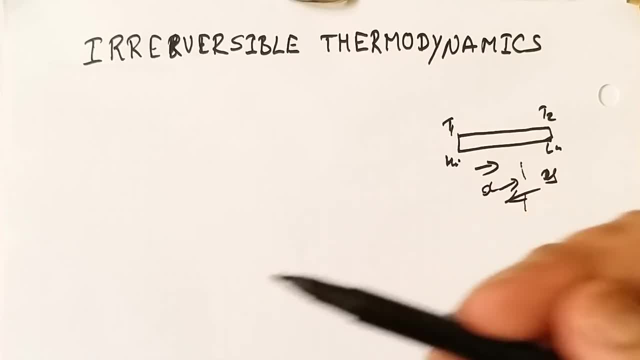 certain additional postulates which has to be introduced, and this postulates: they are applicable only to the system which are not too far away from the equilibrium. so they are applicable only to the system which are not too far away from the equilibrium. so they are applicable only to the system which are not too far away from the equilibrium. so they are. 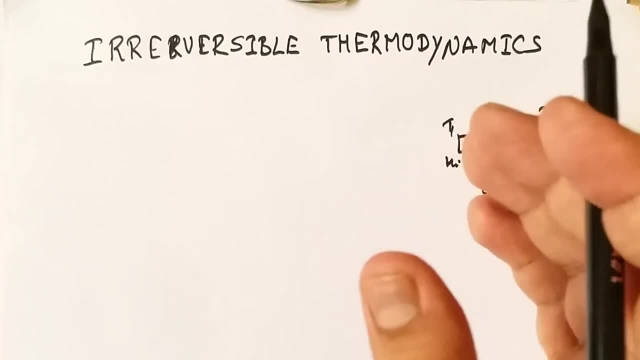 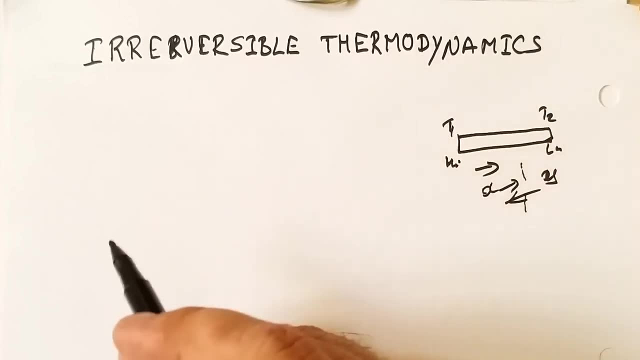 applicable only to the system which are very near to the. we are very near to the equilibrium, or we may say that all the systems which passes through a pseudo equilibrium or which passes through a false equilibrium. so this irreversible thermodynamics is applicable to all those processes. so moving on. so this is the definition and the introduction, and we have seen few examples. 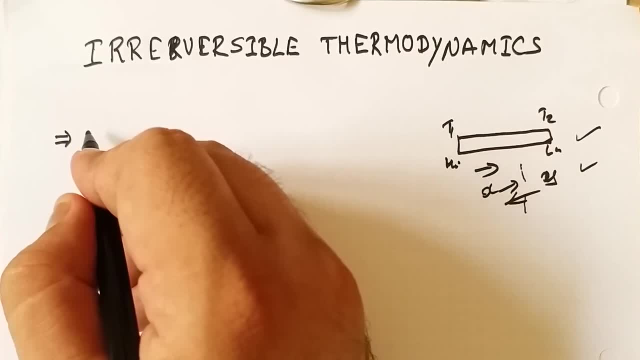 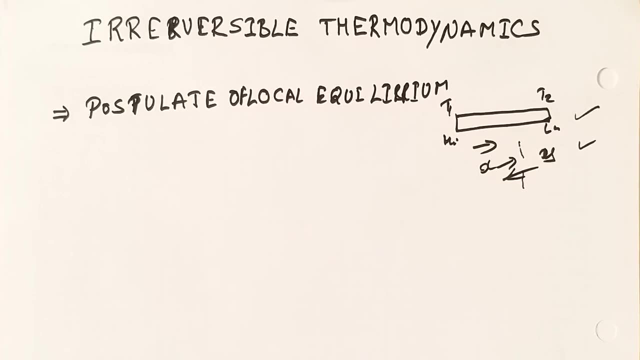 of irreversible processes. now, moving on to the next point, and that is postulates of local equilibrium. this postulate defines the local equilibrium, or it tells us that what type of or where our, when, our system will be under local equilibrium. so for this, in order to understand this particular phenomenon, suppose we are taking a particular 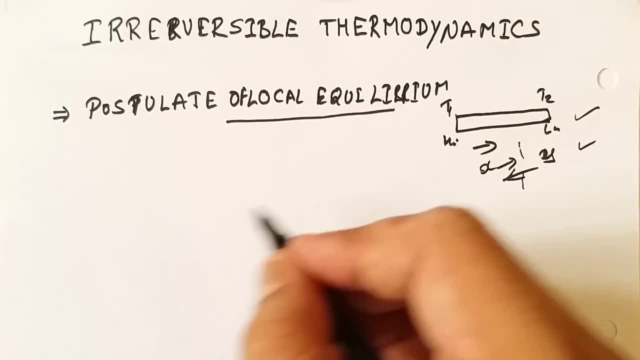 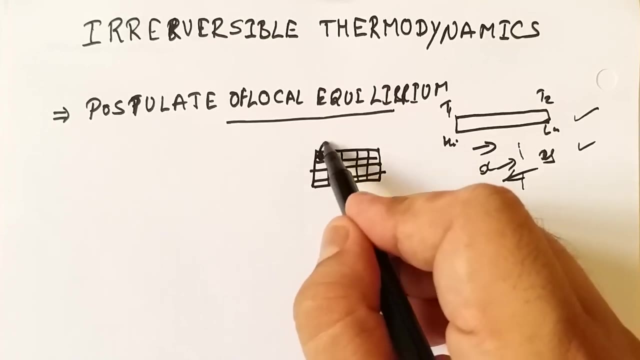 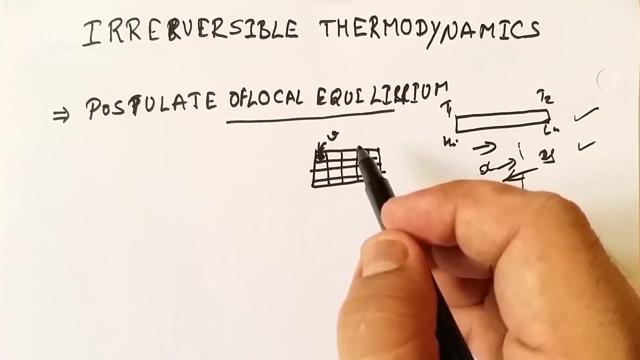 system and that system is divided into small elements. so suppose we have a particular system and this system is divided into smaller elements, likeén some parts of system比 divided into very small elements of volume V, so each small element. so this is one small element whose volume is V and this volume is fixed. now this, now it. 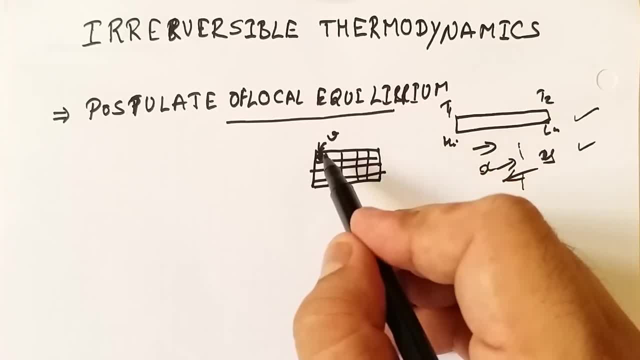 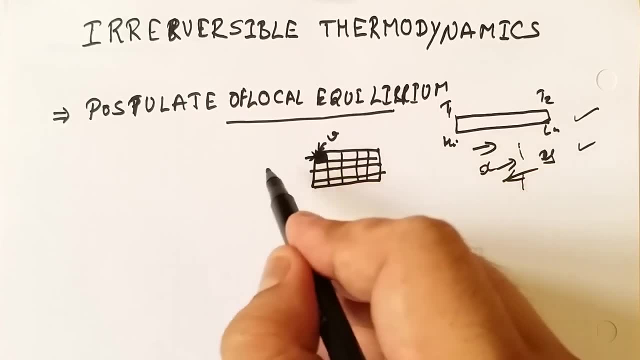 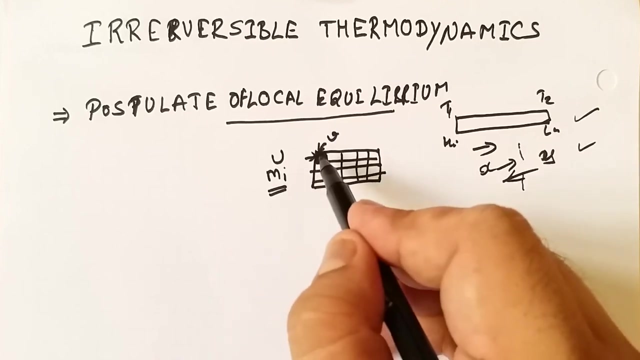 is further said that at any instant time, this particular set or this particular small element, it will have certain amount of internal energy, U and certain. suppose we say that mi is the mass per unit, volume or mass, yeah, mass units of the molecular species. okay then, when this system is under equilibrium, then at: 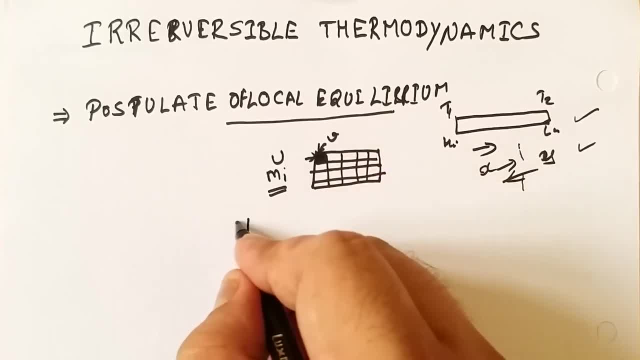 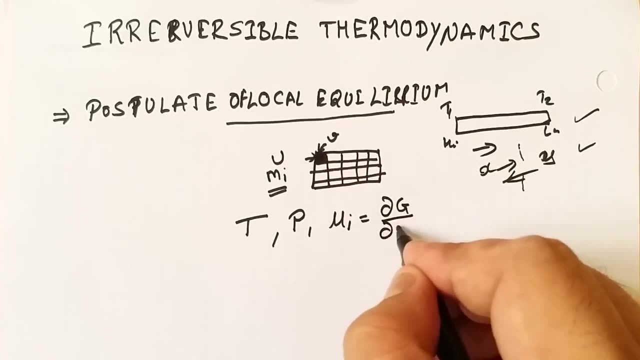 equilibrium, the temperature at equilibrium, the temperature pressure and the partial Gibbs function, or partial Gibbs function, or we may write it as our chemical potential, and that is dg upon dmi at constant temperature and pressure, and the last term, that is entropy. so all this paramit, all these parameters, they are also a constant as 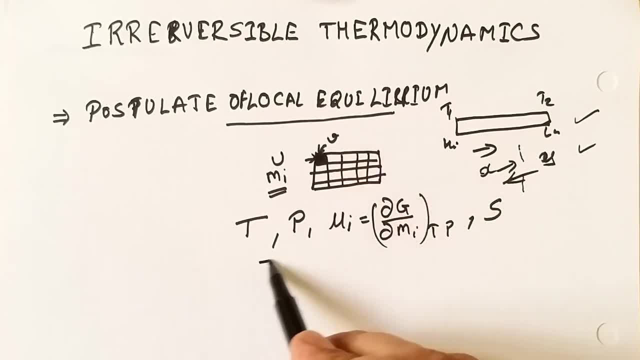 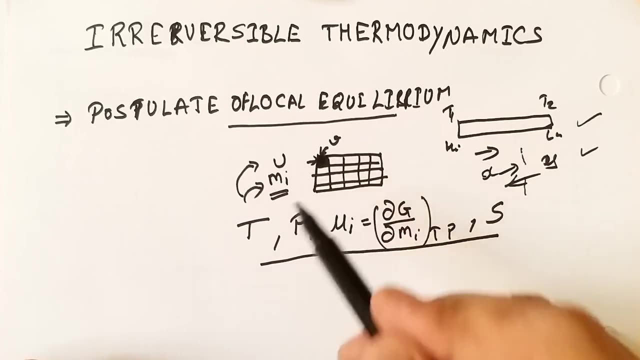 the volume of the system is constant, and all these parameters can be determined by, say, either internal energy or a mass mi of the system. okay, at when our system under equilibrium? this was the case when equilibrium exists. if equilibrium does not exist, then it will be necessary, or when equilibrium does not exist, it will. 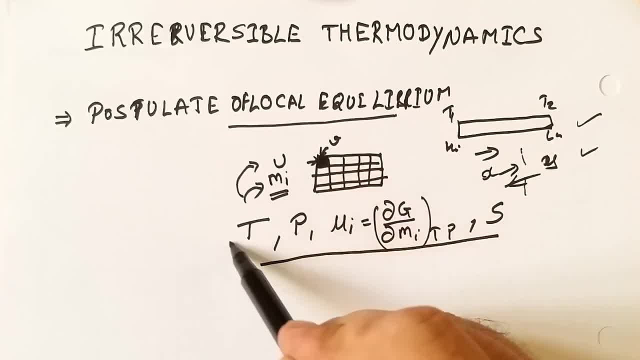 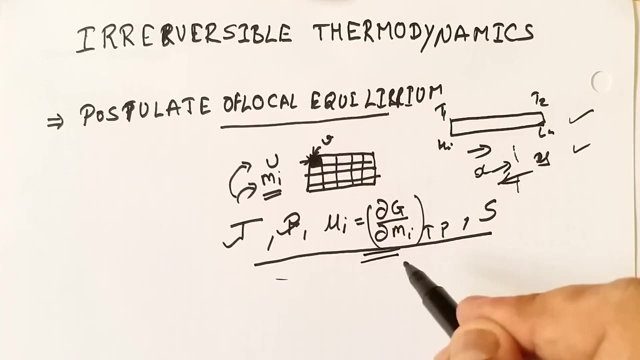 be necessary to redefine the temperature pressure and all these terms. okay, and hence it is assumed that the temperature pressure, specific temperature pressure and the specific Gibbs function and entropy for the cell in a non equilibrium state it depends. so in non equilibrium state also it depends on the internal. 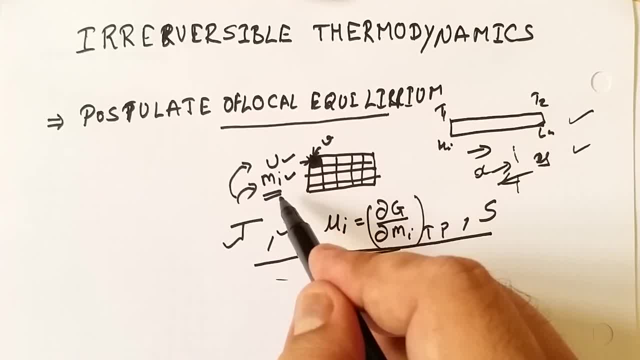 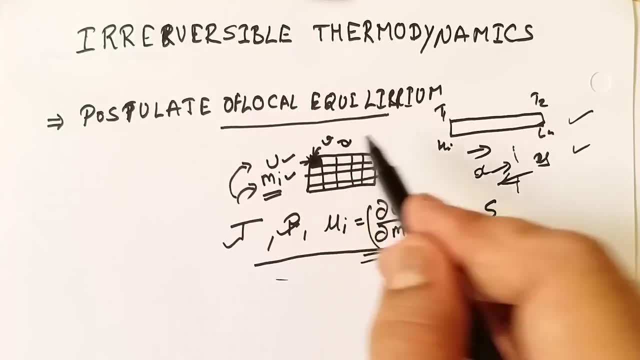 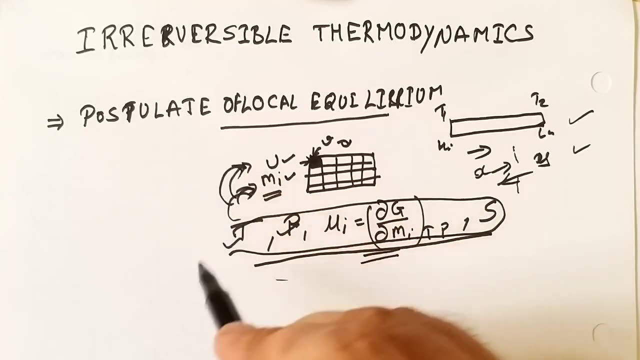 energy and the mass unit of the system of the molecular species, exactly as it was depending on when our system was under equilibrium. so when our system was under equilibrium, then also all these properties were depending on both these things. and when our system is not not equilibrium, then also all these properties. they are. 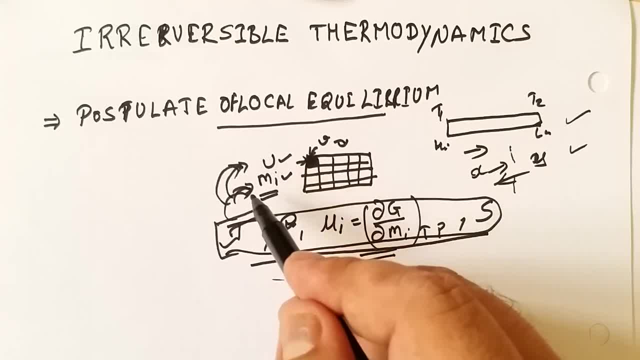 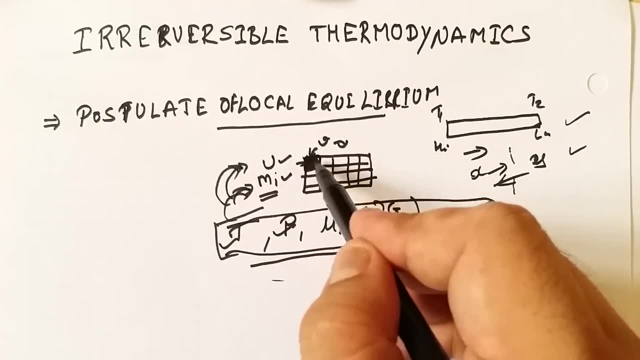 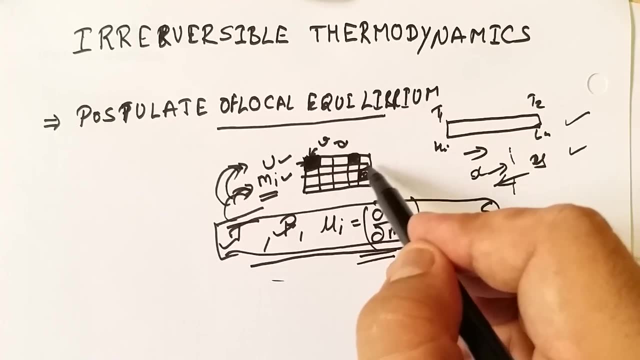 depending on both these, as it was depending on when it was in equilibrium situation. so in other words, we may say that for a non-equilibrium system, each of the cell- okay, that is, each of this particular cell- is each of this particular cell- is the treated exactly in the same manner as if that equilibrium exist in. 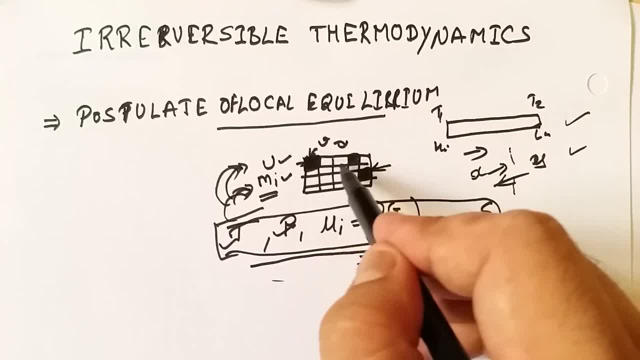 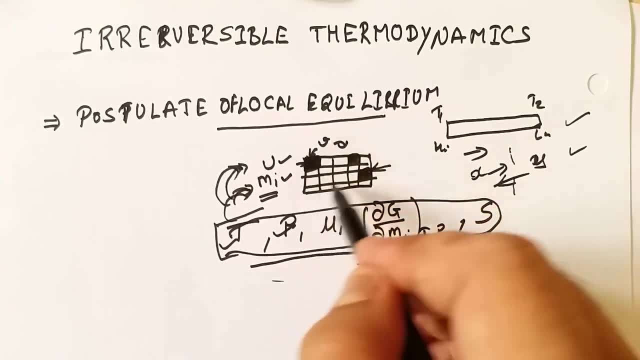 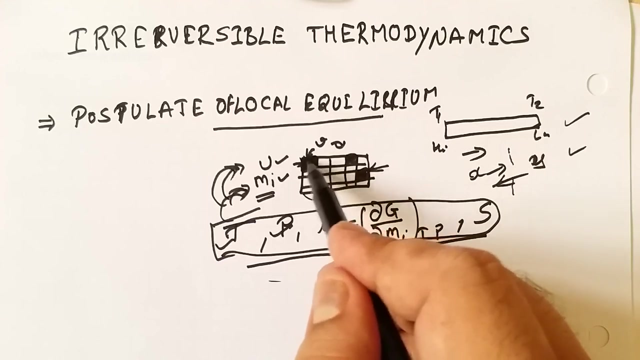 this particular cell. so we are looking at the equilibrium of the individual cell and we are not looking at the equilibrium of the whole system. so this assumption is treated as local postulate of local equilibrium. so in postulate of local equilibrium, basically we are considering that the individual cells are under non-equilibrium condition. the system is divided into large number. 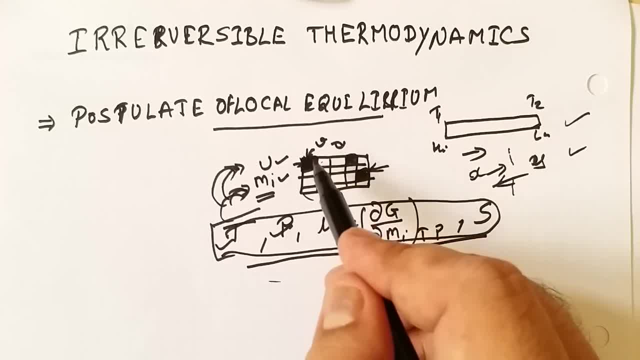 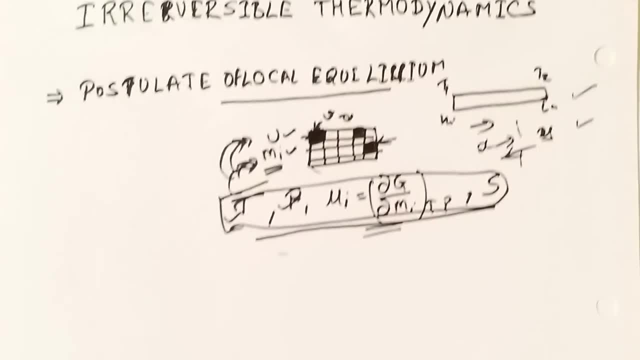 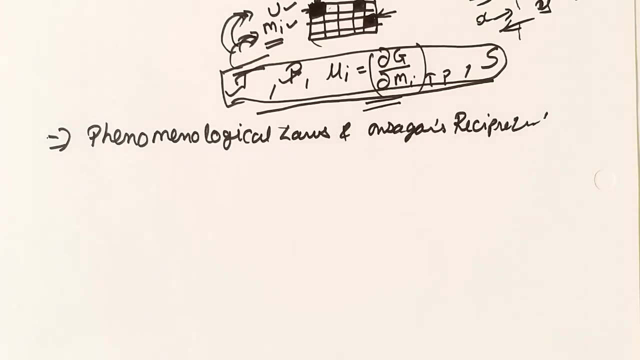 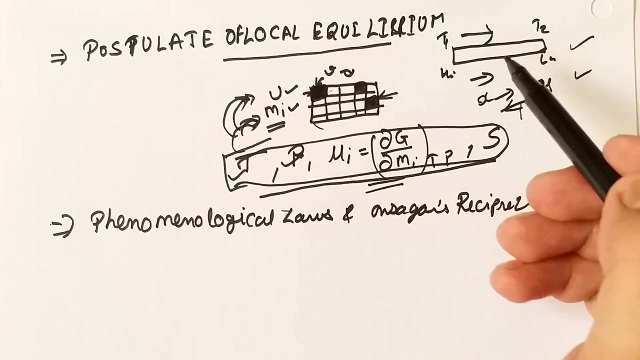 of individual cells and each individual cell is under equilibrium. so that is the basic postulate of our non-equilibrium, postulate of local equilibrium. okay, moving on to the next point, that is, phenomenological phenomenological laws and onsager's reciprocal- we have seen that- irreversible thermodynamics, they consist of several transport phenomenons. okay, and basically, 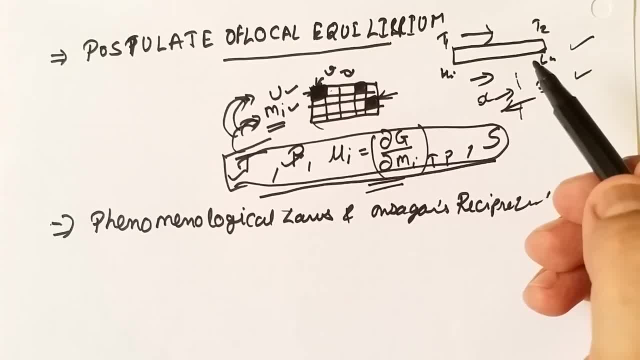 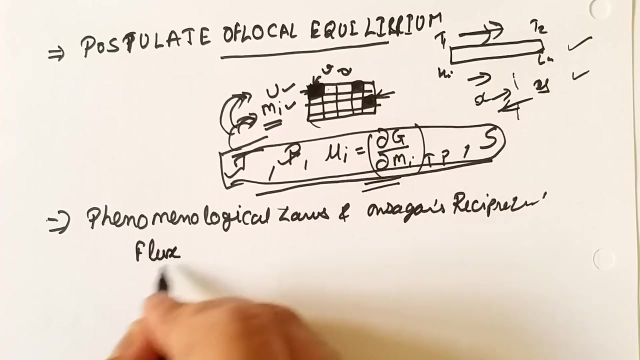 all these transport phenomenons are basically a one-dimensional system, that is, they move along only one axis or they are one dimensional system. so there are several quantities, like we have heat, mass, momentum, electrical charge, etc. okay, now this quantities, this quantities- they are particularly referred as fluxes. okay, that is, we have heat, we have mass, then we have momentum. so 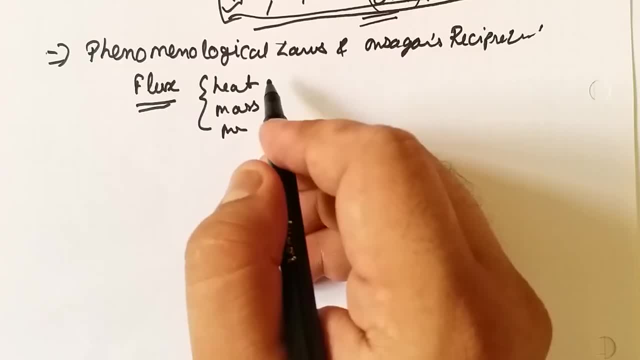 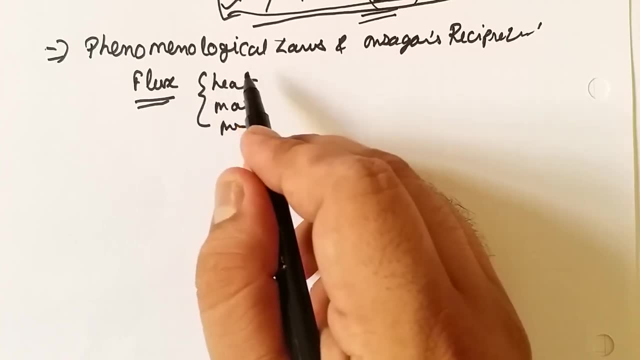 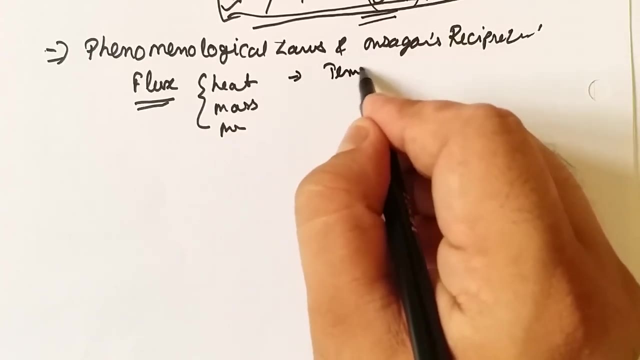 these quantities- they are referred as fluxes- and there is a driving force because of which these properties are generated, so that is known as the driving force. so for heat, we know, the driving force is the temperature gradient. okay, it is temperature gradient. and then for mass it is. 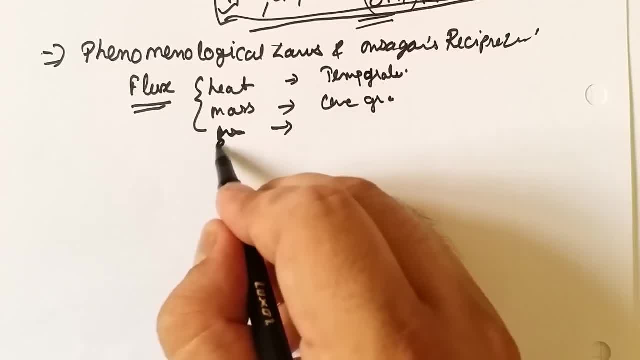 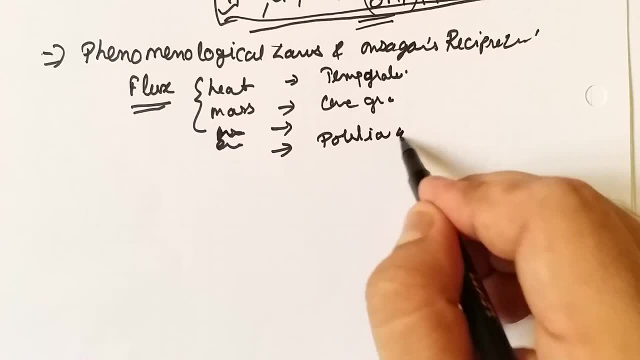 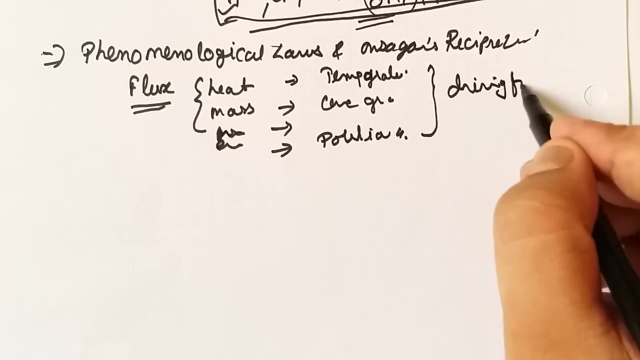 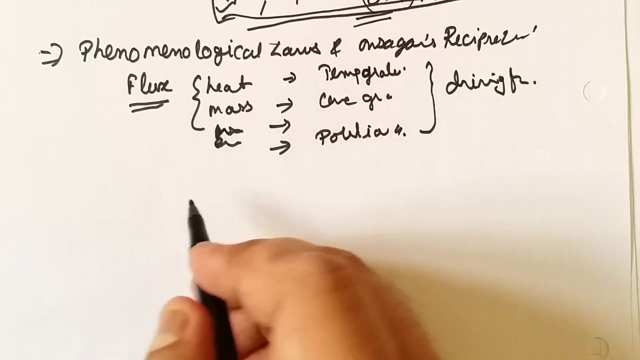 concentration, concentration gradient for electricity. for electricity we know it is the potential, it is, it is potential gradient. so for any particular force there are different types of, there are different types of driving force. so we may write that this fluxes, they are directly proportional to this direct, they are directly proportional to this driving force. so suppose 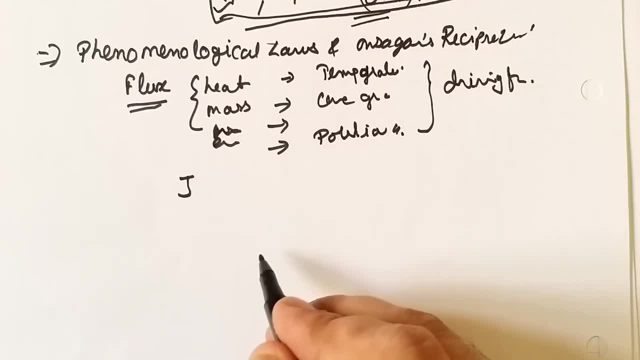 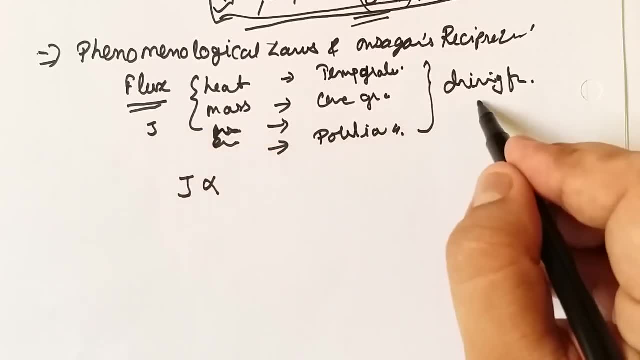 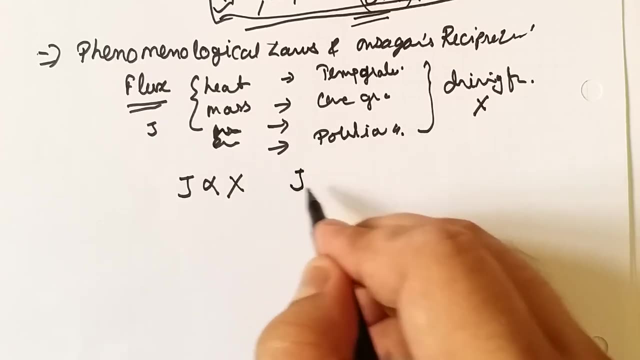 if we consider that j is the flux over here, then this flux j will be proportional to the driving force. and suppose, if we write that x is the driving force over here, so we may write that j is proportional to x and hence we can write that j in order to remove the proportionality sign, we may write: 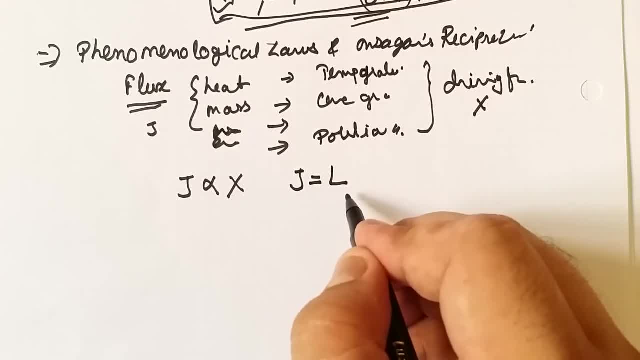 any proportionality constant. and suppose we write that l is the proportionality constant over here which is called as transport coefficient, then we can write: j is equal to l into x, so over here j is our flux, then l is our transport coefficient and x is our driving. 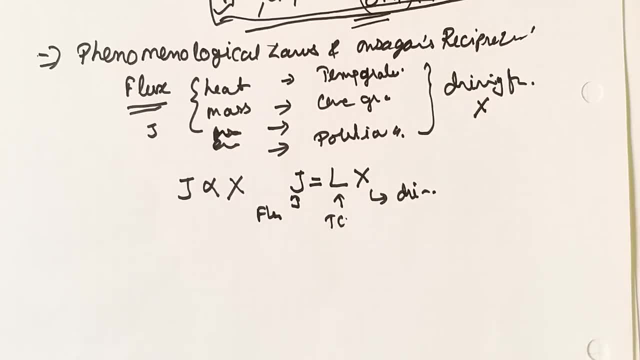 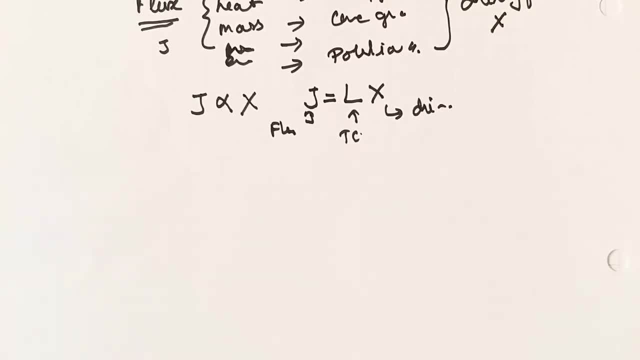 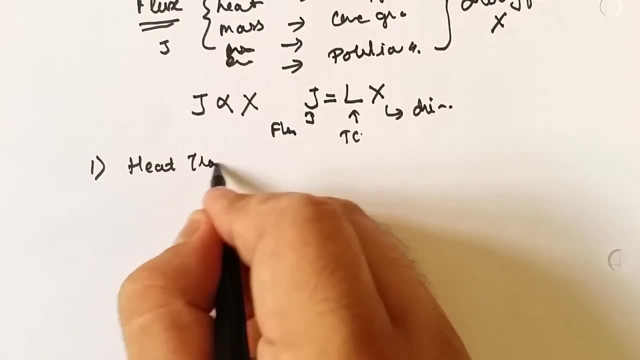 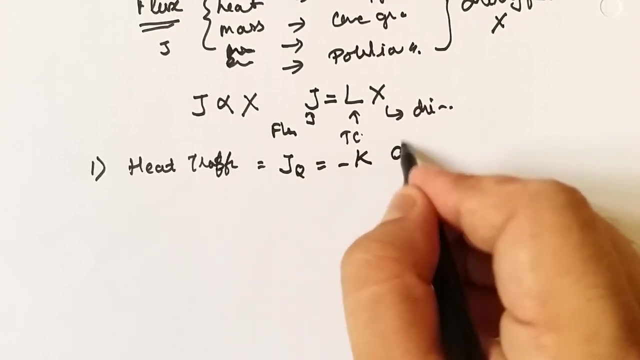 force. okay, so based on this particular assumptions, uh, various transport phenomenons or various expressions have been given for several transport phenomenons. so the first transport phenomenon, and that is suppose, if you consider that heat transfer, then for heat transfer we can write that j is equal to minus kappa, dt upon dx. okay, where jq is our heat flux, then k is the. 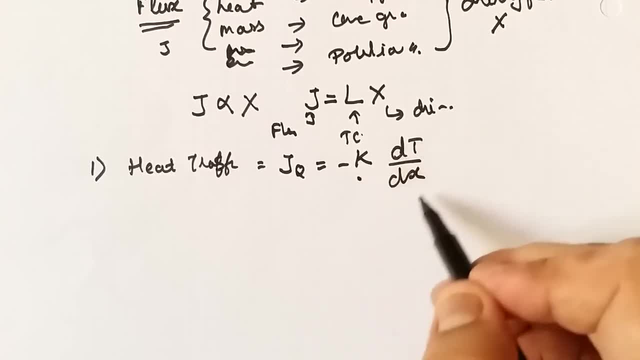 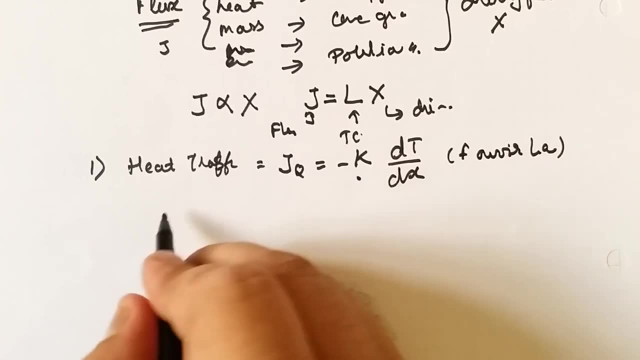 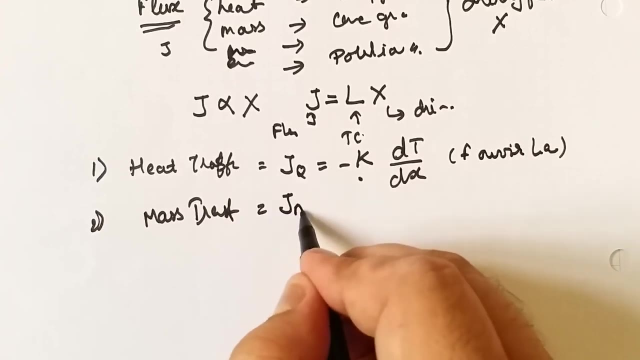 transport coefficient and dt upon dx is the rate of change of temperature. so this is also known as our uh fourier law. similarly, for mass transfer. for mass transfer we can write: jm is equal to minus d dc upon dx and this is our uh fixed law of diffusion. so this is the fix of diffusion. 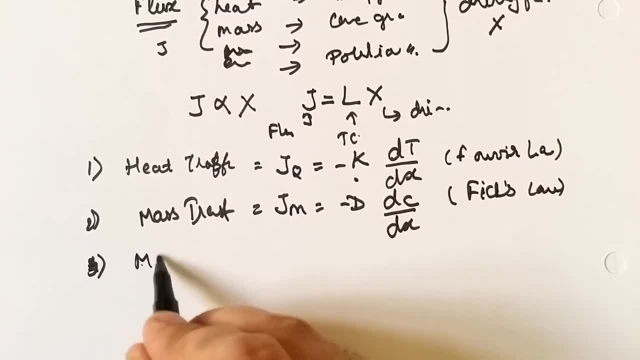 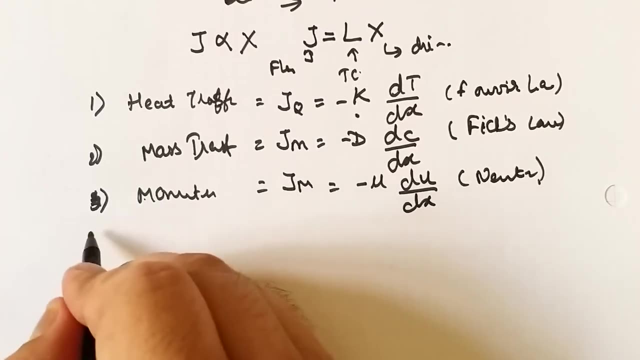 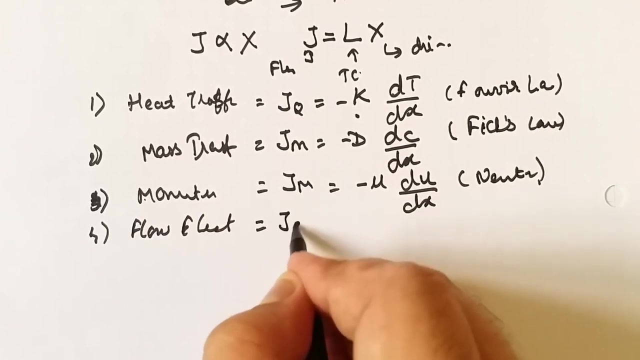 similarly for uh, momentum transfer. for momentum transfer, we can write j. capital n is equal to minus mu du upon dx. so this is our newton's law. basically, this is the second law of newton and the third law is our flow of electricity. flow of electricity, and that we can write it as j. 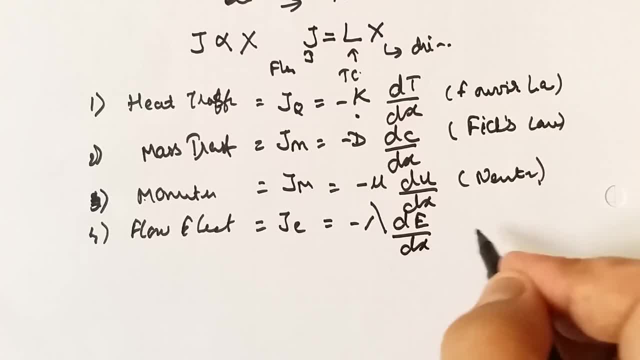 e is equal to minus lambda d e upon dx, and this is our ohms law. so, over here, all these are the fluxes and these are the driving force, that is the gradient because of which we see this particular flux and this kappa d mu and lambda, they are the transport coefficients and this 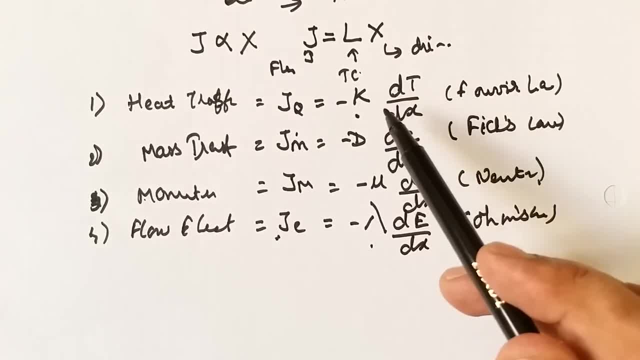 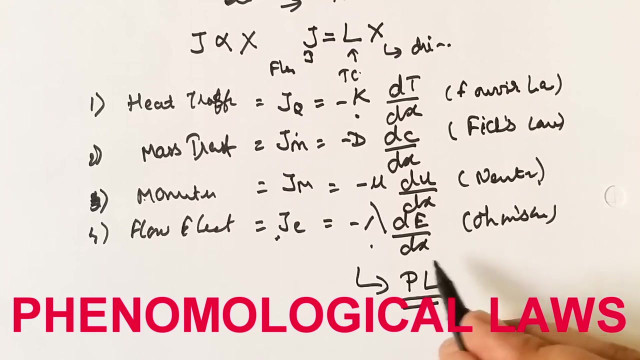 coefficients. it depends on the properties of the material of the system that we have taken. so all these, they are basically the expressions which are taken in use and there is no particular derivation for this expression. and all these expressions are known as the phenomenological laws, which are used or which are used to define several transport processes. so all these, 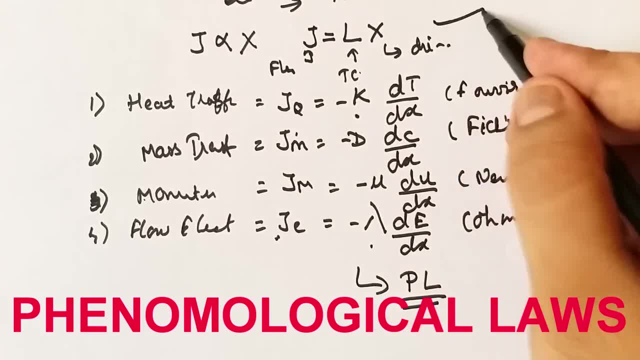 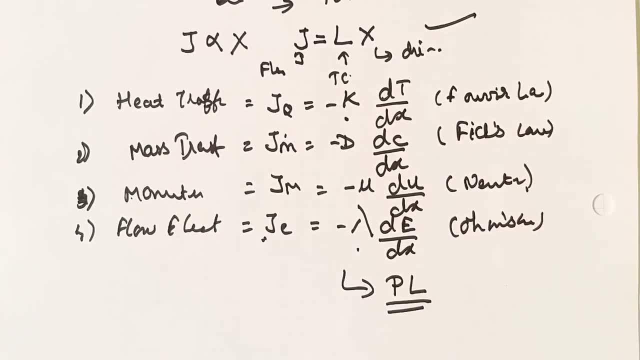 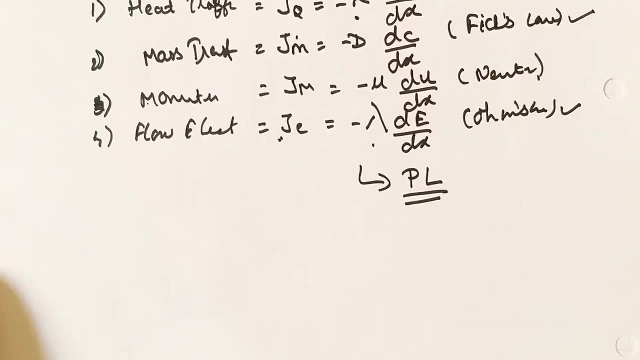 expressions are engine. the general term, that is j, is equal to l into x. they are known as the phenomenological loss. okay, and over here, amongst all these phenomenological laws, the ohms law, as well as the flix law of diffusion, they are some of the familiar example that we are looking into. for 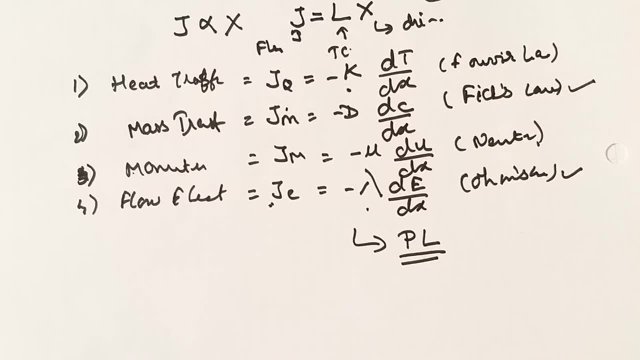 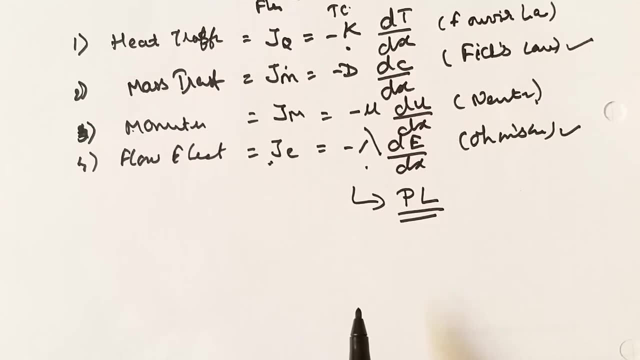 several particular times now, when we look at this particular phenomenological laws, or this phenomena, the logical laws. basically, it describes the irreversible thermodynamics of a particular system. okay, now we will move further by taking, or by taking the example of our fix law of diffusion. now, when we are looking at a simple 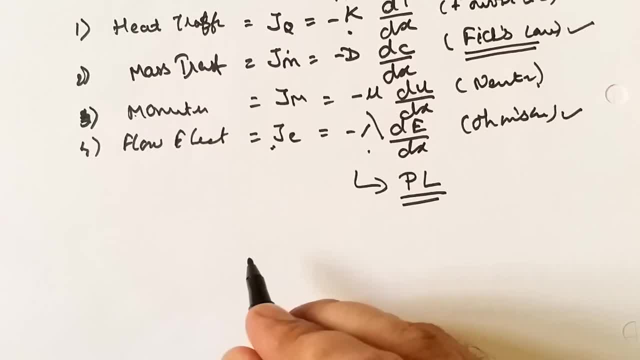 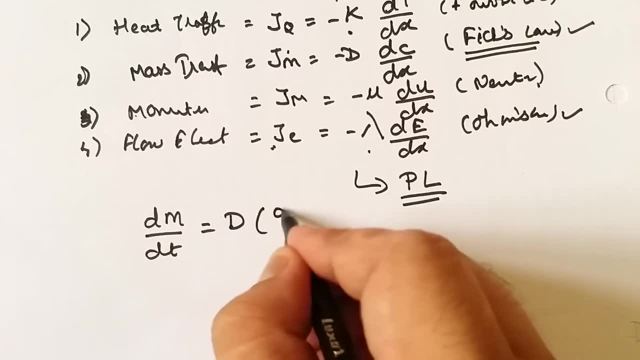 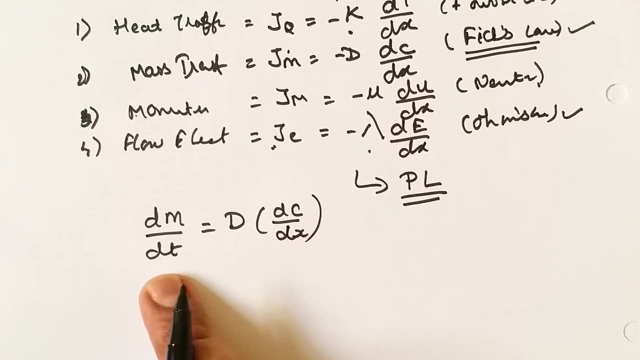 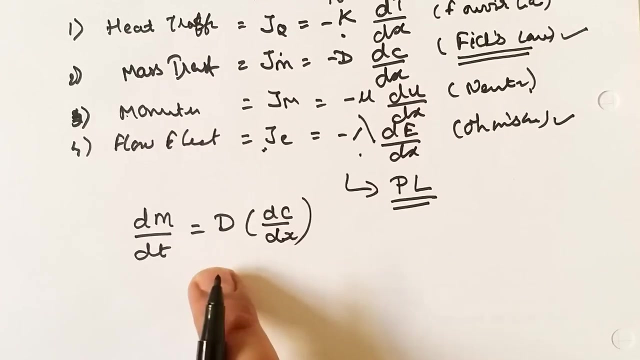 one-dimensional system. then for a simple one-dimensional system, suppose we can write the expression, as dm upon dt is equal to d, into dc upon dt upon dx. so dm upon dt over here is the rate of change of the solute across the surface and dc upon dx is the concentration gradient and d is the diffusion coefficient. so particularly, 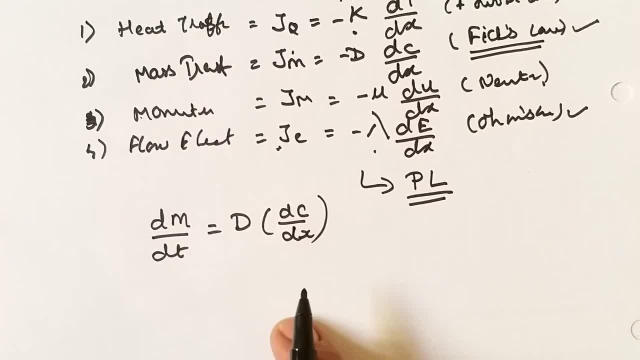 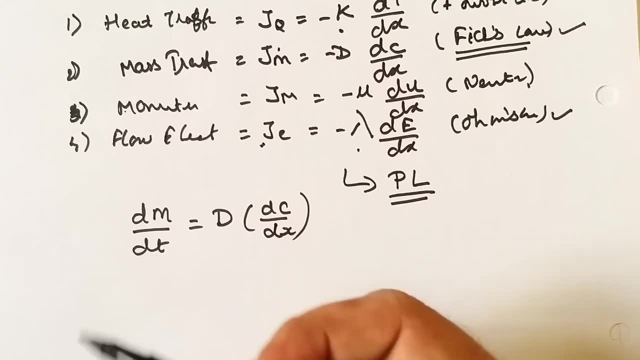 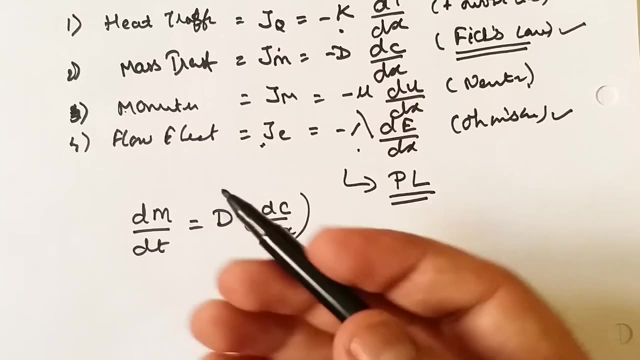 what we are looking at is that we are having a system, or suppose- let us take an example- that we are looking at an osmosis process. so in case of an osmosis process, the solute from lower moves towards higher concentration. and suppose we are performing osmosis, then under or when we are, 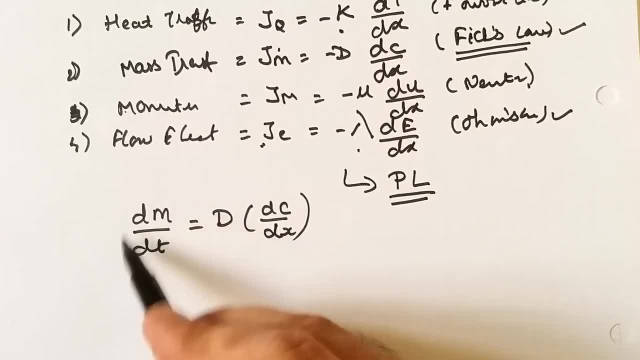 performing the osmosis, we say that dm upon dt is our rate of change of the solute, or it is the rate of change of solute uh which is moving across the surface. then, and dc upon dx is the concentration gradient on both the sides of our the semi-permeable membrane that we have taken. okay, so 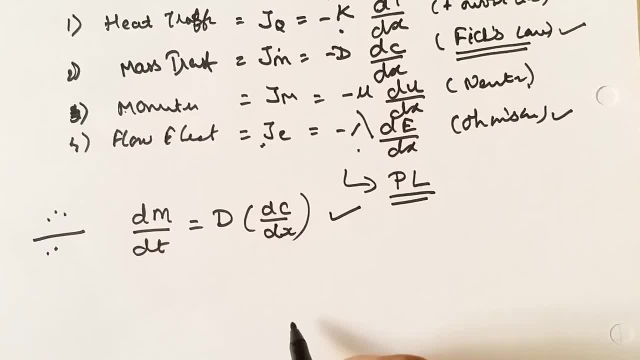 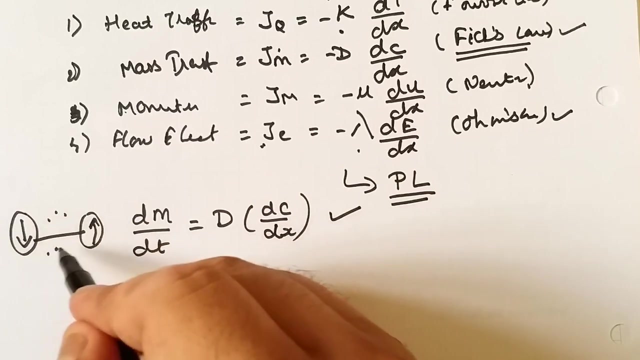 this expression is sufficient for explaining the single, single system now. so along with this particular thing, uh, one more phenomenon may take place: the diffusion or the concentration gradient, the moment of solute from, say, one side to other side will take place. also from other side to one side will take place. that means that concentration of the solute and the solvent 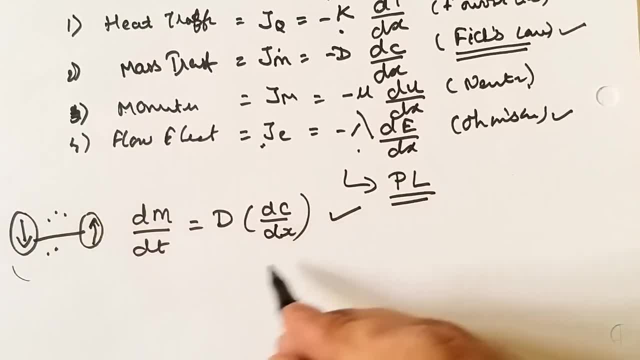 they are moving from both the sides. so hence us, is this statement or is this law of sufficient to explain both the phenomenons? one more thing: that with the change in the concentration gradient there exists also a temperature gradient. that means there will be a variation of temperature also along with this change in the concentration. so is this: 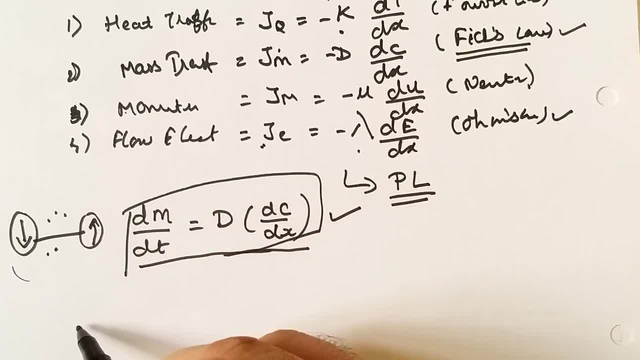 expression sufficient to explain both this. so the answer, obviously, is no. so we need to change or we need to modify this particular expression which can explain both the systems, that is, which can explain the temperature change also, or temperature gradient also, and which can explain the concentration gradient also. so suppose, if you are considering that we are looking at a 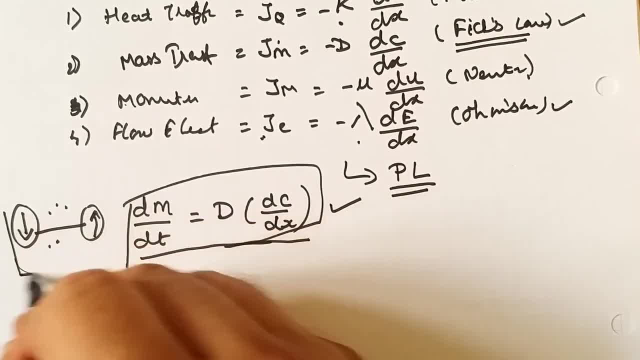 concentration gradient, that is, change of concentration from one side of semipermeable- suppose this is our semipermeable membrane- so the solute will flow from here to here and here to here. solute is moving from both the sides. okay, so the generalized expression for this particular system, wherein: 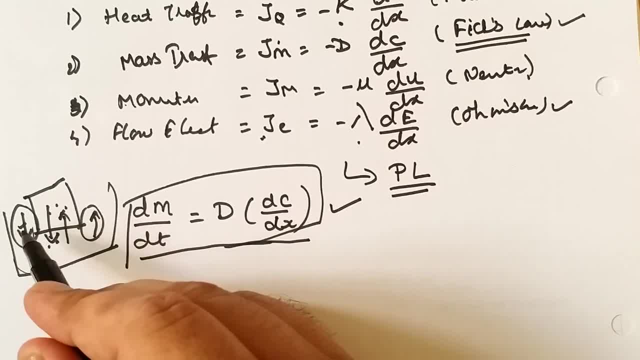 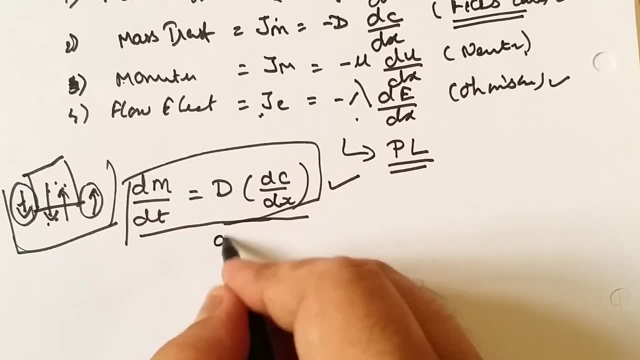 the solute or wherein there is a change in the concentration gradient from both the sides, that can be written. as for the first system, we may write it as dm1 upon dt, that is equal to dc1 upon dx plus e into dc2 upon dx. so over here. 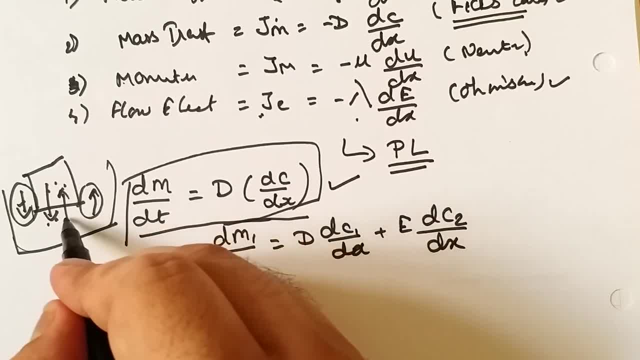 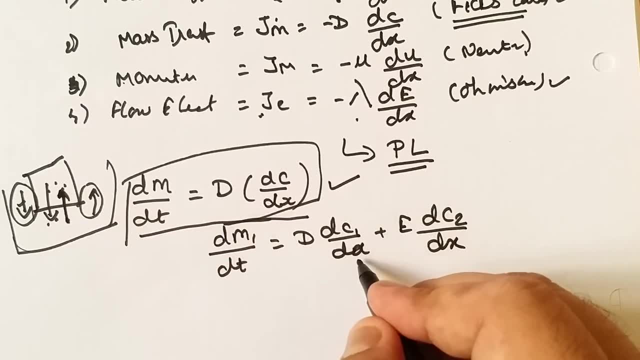 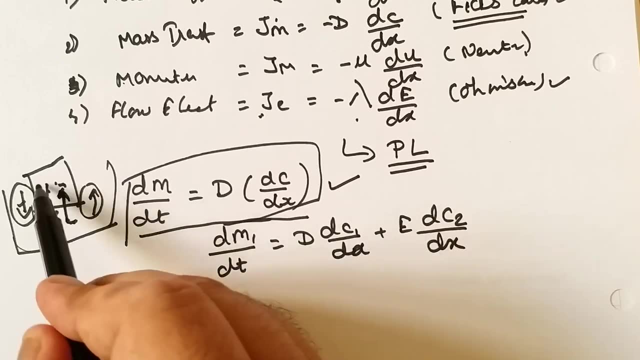 dm1 upon dt, it is the moment, say suppose moment of concentration gradient from here to here, and dc1 upon dx is our concentration gradient of first solute, said that is a concentration gradient here to here, and dc2 is from here to here and dn e are the constants. and similarly for the second system. 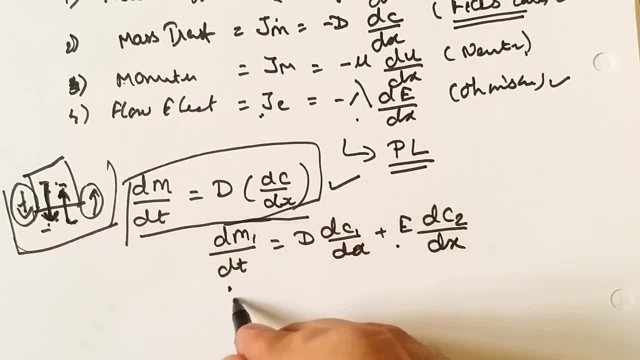 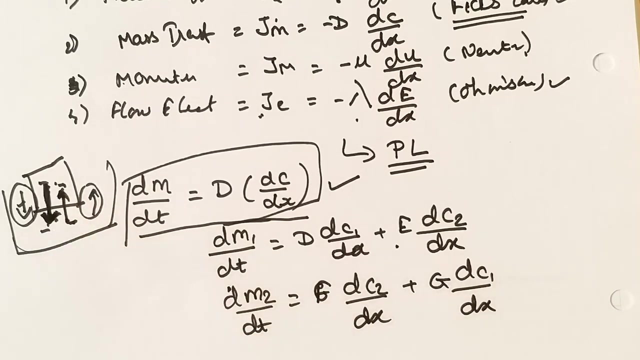 that is, when the concentration gradient is moving from here to here. the expression can be written as: dm2 upon dt is equal. to suppose this is our f, dc2 upon dx plus g into dc1 upon dx. okay, so this will be our second expression when we are considering that the concentration is moving from here to here. okay, 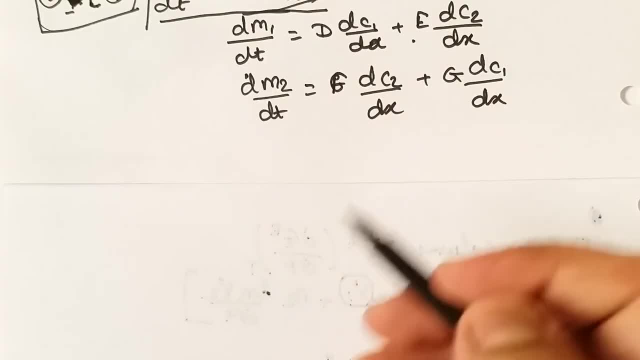 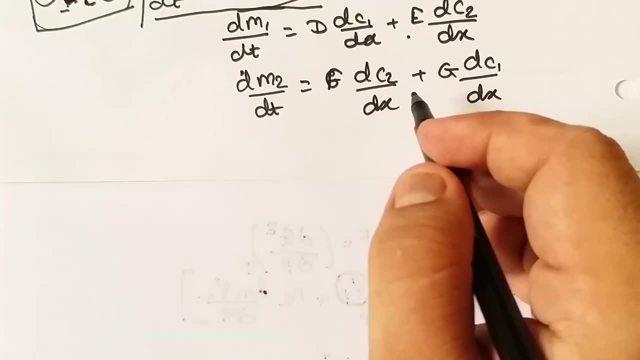 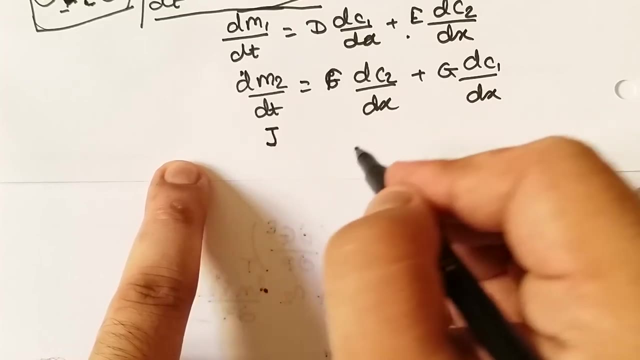 so these are the expressions and now, in order to simplify, uh, this particular notation, okay, we are considered again, considering the same thing. uh, that we are considering the same thing and that is why we are using the啊 and we are using the. have considered that for a particular flux, suppose we are writing J is the flux over? 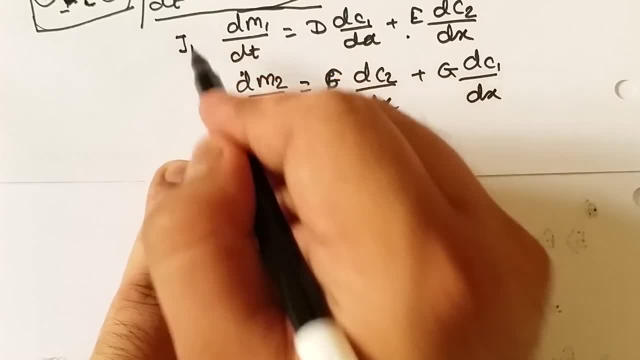 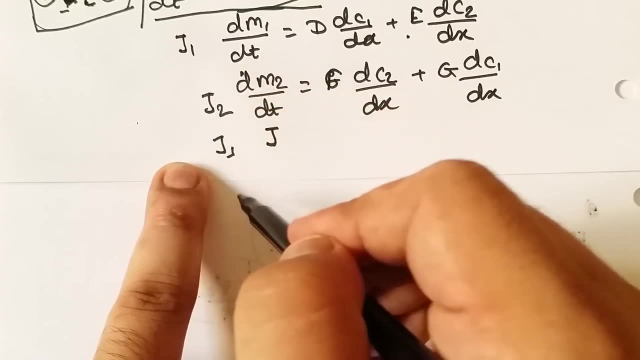 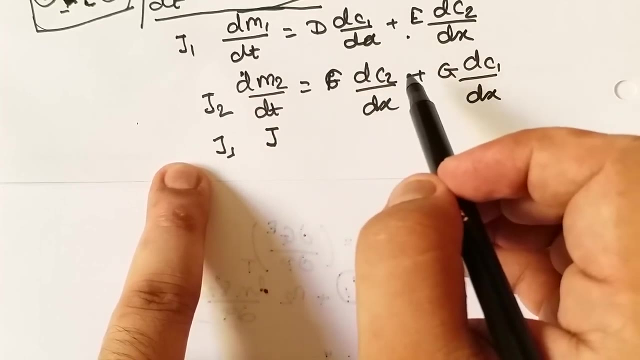 here. so for m1 we will have j1 and m2 we will have j2. so, similarly, if there are three things, then we will have j1, j2, j3 and so on. okay, and this coefficients, that is d, e, f and g, this coefficients, they are replaced by, suppose coefficients. we know coefficients are written. 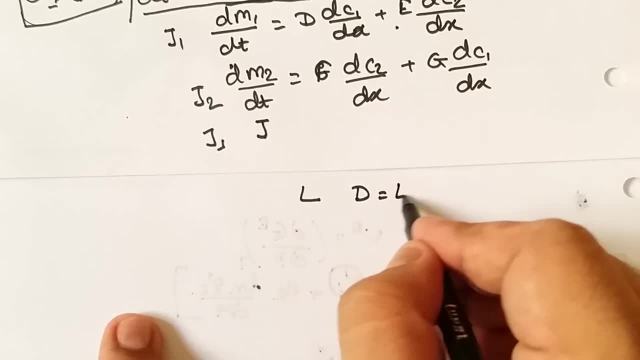 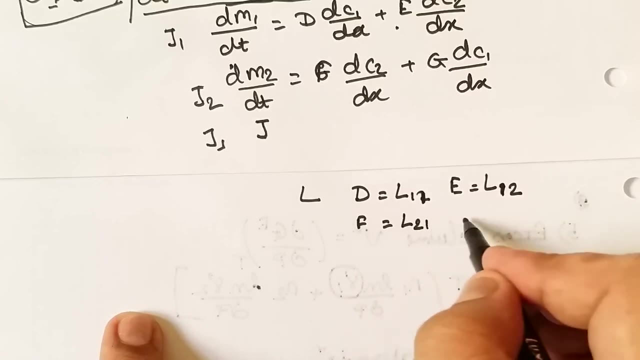 as L, so we can replace d is equal to. we can write L12. then, similarly, e is equal to L, sorry, L11, and this will be L12. and similarly, f will be equal to L21 and g will be equal to. f will be equal to sorry, it will be L22, and g will be equal to L23m1, so we will have k1k1k1k1. sorry, it will be l22 and g will be equal to. they will be same, so you can write E as quote. next action, ration can replace: d is equal to 1l1. c'll be Io, right, so can you give. Cq is evenly different. the según küçük sui n, m2 and the Q1 will be equal to v1n2. Sorry for M1, right, so? 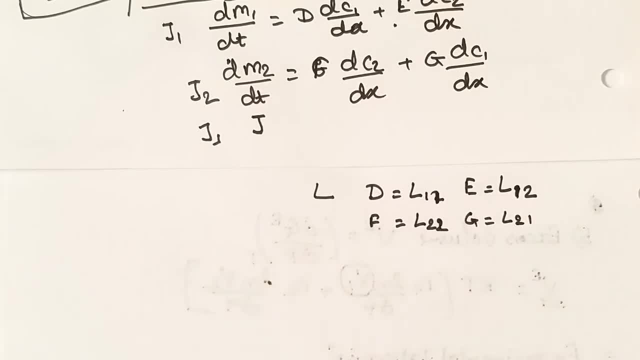 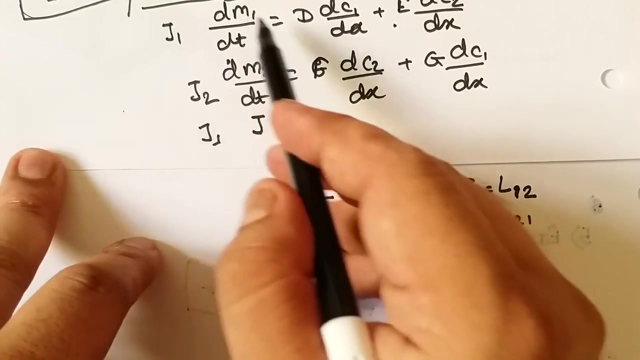 to l to 1. okay, so over here, and this will be the coefficients, we can write l and this subscripts it. the first subscript: it refers to the component that moves, and the second subscript it refers to the component whose gradient is being considered. so over here in m1, we are considering. 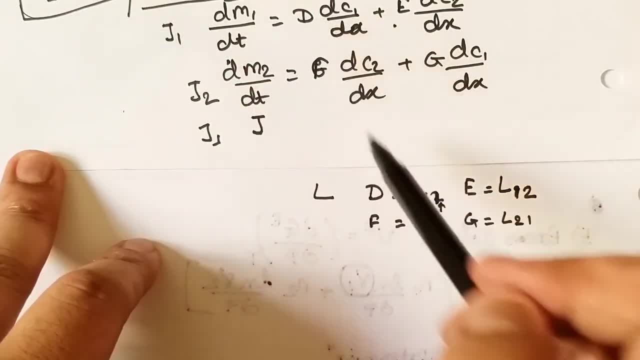 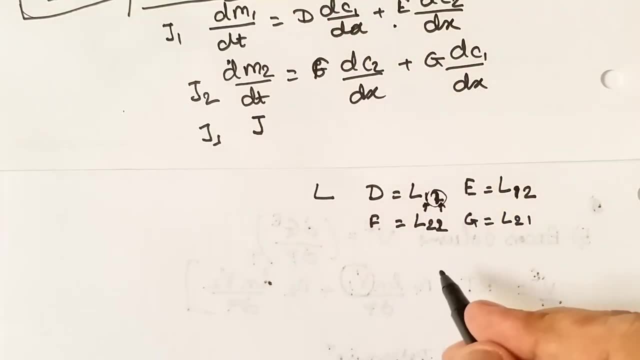 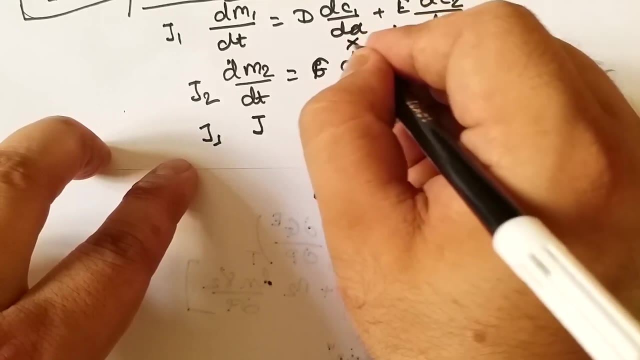 that it is moving from here to here, so we will have c1 and hence, and the other gradient, that is 2, is considering that concentration. we are considering the concentration gradient, okay, and similarly the driving force, that is, this is the driving force, so driving force, we can. 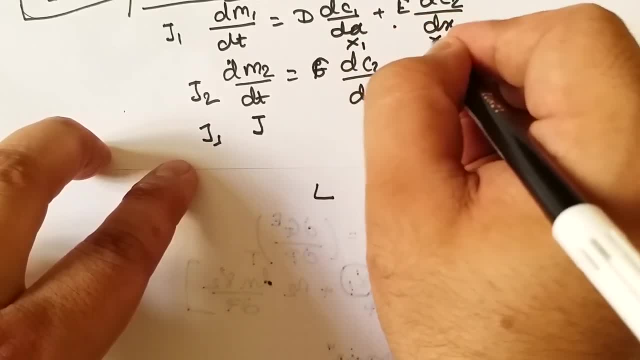 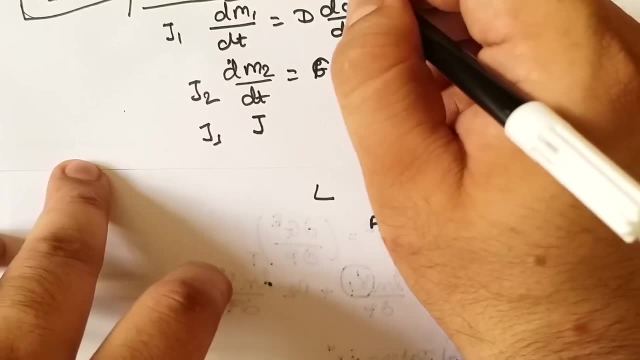 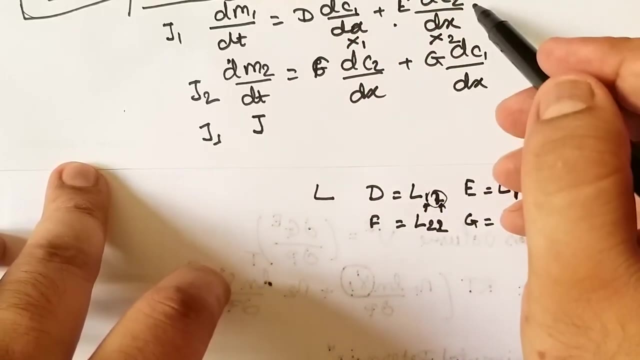 represent it by x. so this will be: we can write it as x1, and this: we can write it as x2. okay, hence we can say that, uh, for a single particular flow, it can be explained for by, or can be expressed by, a single system, while if the two flows, they are independent of each other. 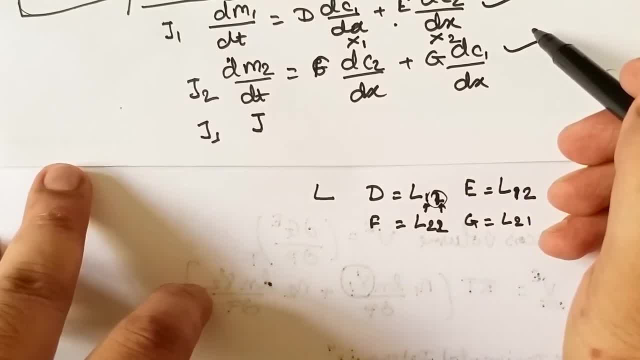 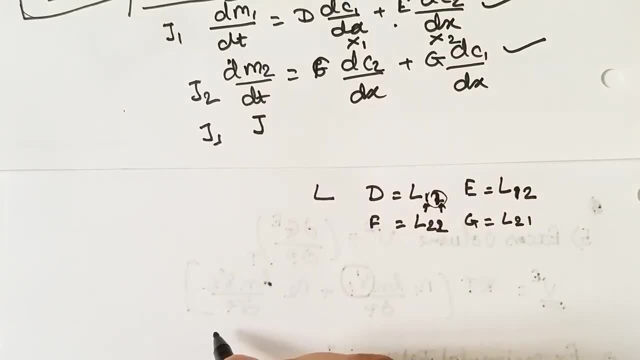 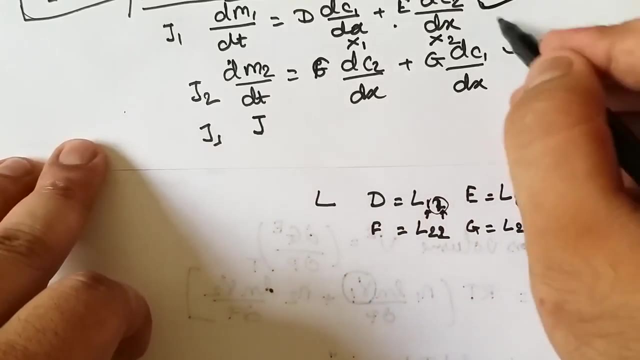 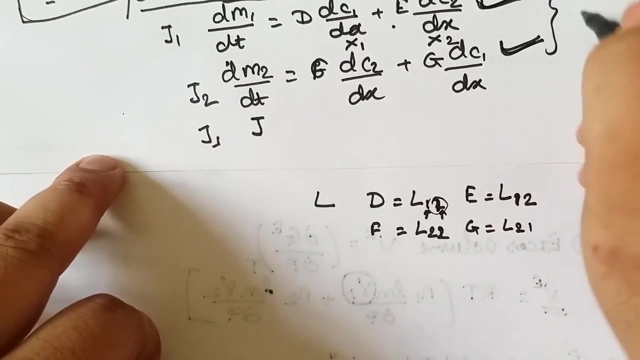 then they can be represented by independent expressions. and similarly, if, however, two simultaneous flows which are not independent of each other's concentration gradients, or which are independent or which are dependent on its concentration gradients, they can be expressed by this particular two expressions and such a flows, which are dependent on each other. they are known as: or they are written or they are. 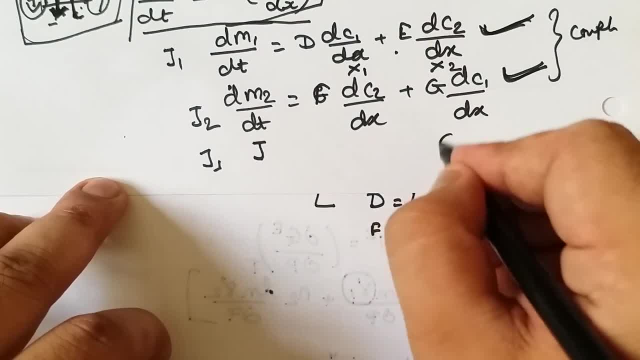 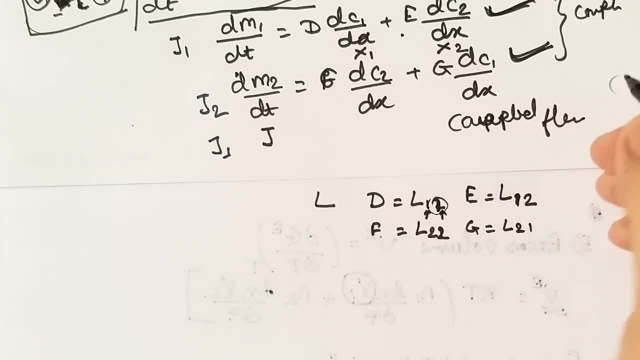 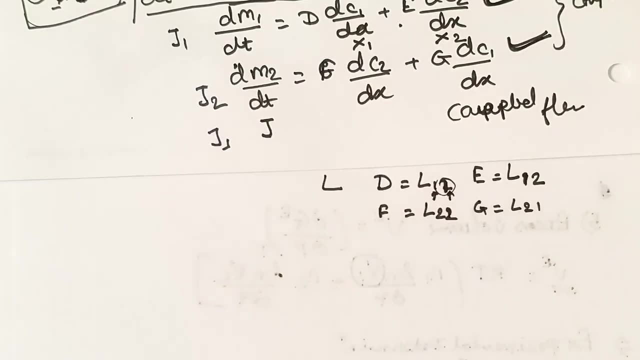 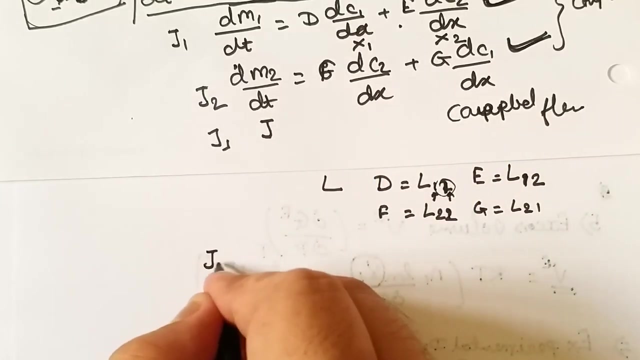 known as uh, they are known as coupled flow, they are known as a coupled flow and once again, he developed an irreversible thermodynamics in 1931 to explain or to explain this type of coupled flows and from this particular expressions, the generalized expression. we can write it as j i is equal to. we can write l i 1 x 1 plus l i 2 x 2, up to: 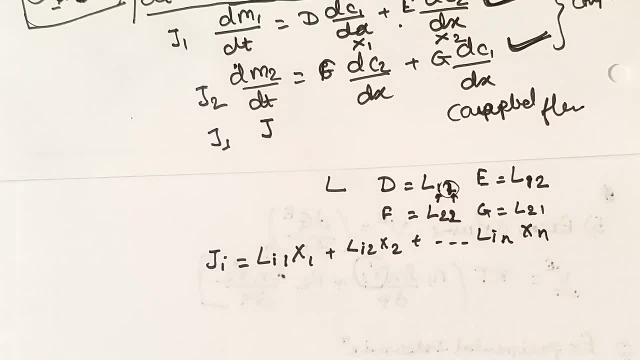 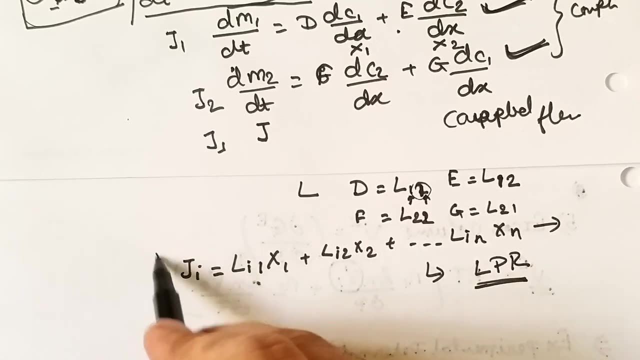 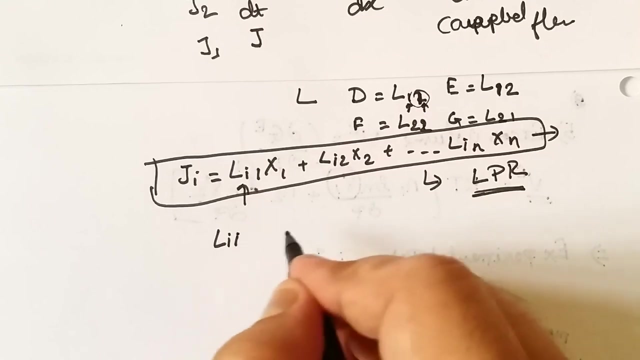 l, i, n, x, and so hence we can write the generalized expression in this particular form and this expression it is known as linear phenomenological relationship, that is, lpr or linear phenomenological relationship. so this particular relationship is known as linear phenomenological relationships. and over here the coefficients, that is, this particular coefficient, that is l, i, i, they are: 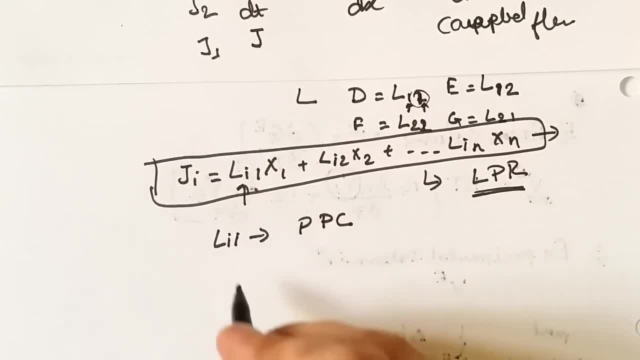 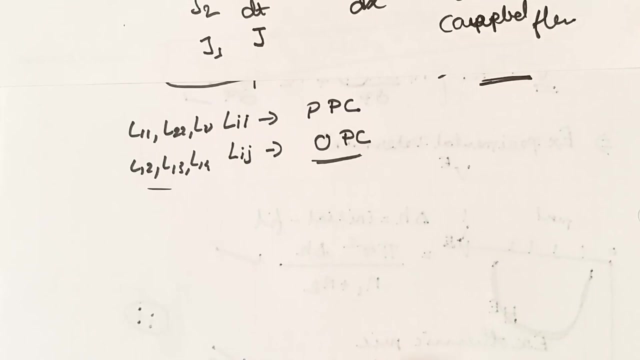 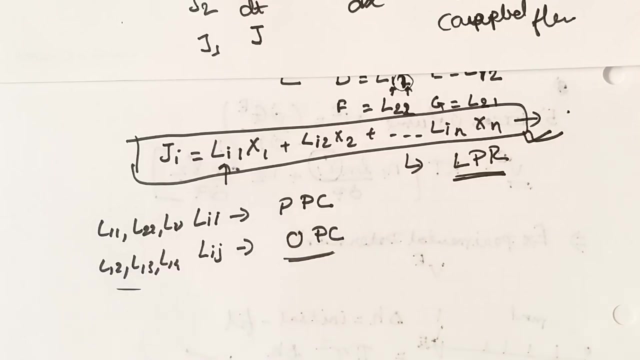 known as primary phenomenological coefficients and the coefficients l i, j. they are known as onsager's phenomenological coefficients. that is, l i. i means l one, one, l one, three, four, l one, two, three in the denominator l 2 will be our primary phenomenological coefficients and similarly, l 1, l1, l 2013. 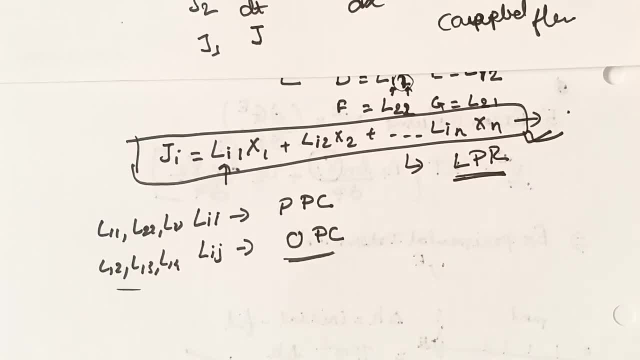 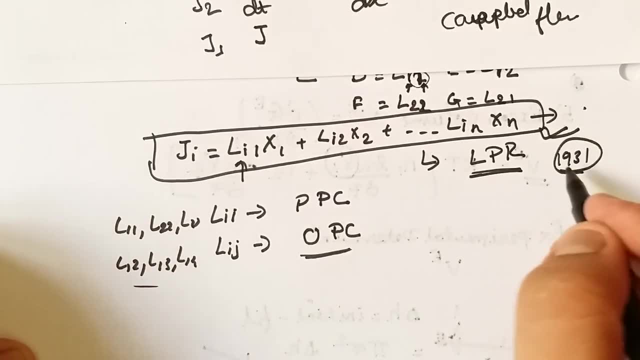 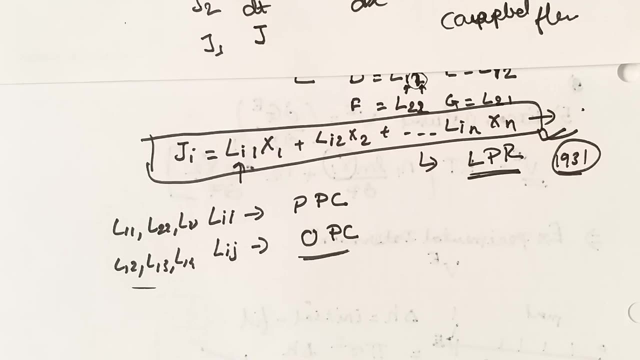 and so on, there will be scientists. they have attempted to solve this expression, however, in 1931, in 1931, once other solved this particular expression. and the difficulty in solving this particular expression, it lies in the fact that the phenomenological coefficients, that is, both this phenomenological coefficients, they have 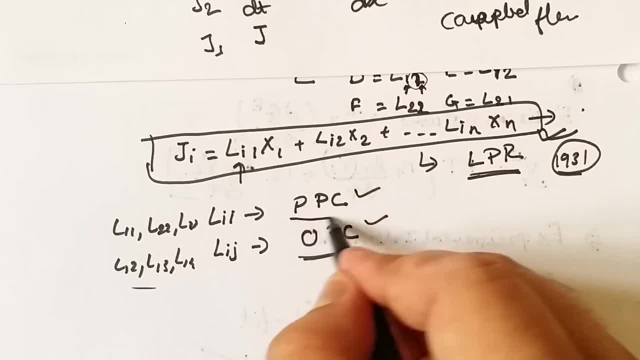 to be determined experimentally okay, and the primary phenomenological coefficients can be determined very easily. but the Onsager phenomenological expressions were very difficult to find out and it requires several control of several experimental parameters to get Onsager's experiment or to get this. 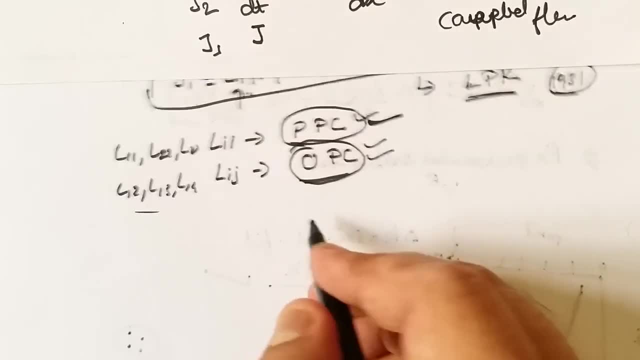 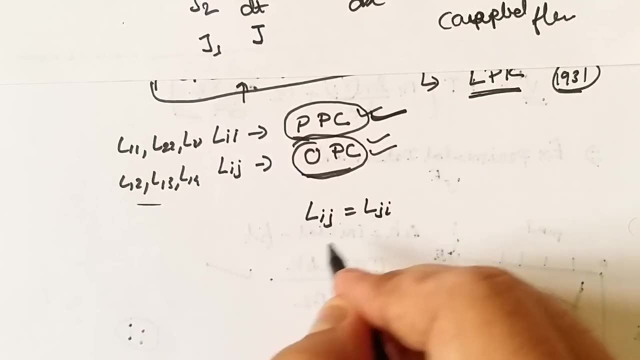 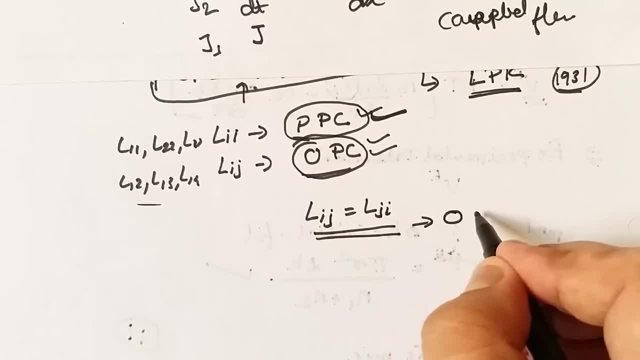 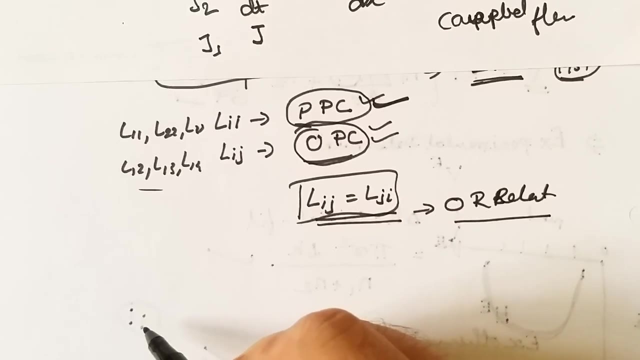 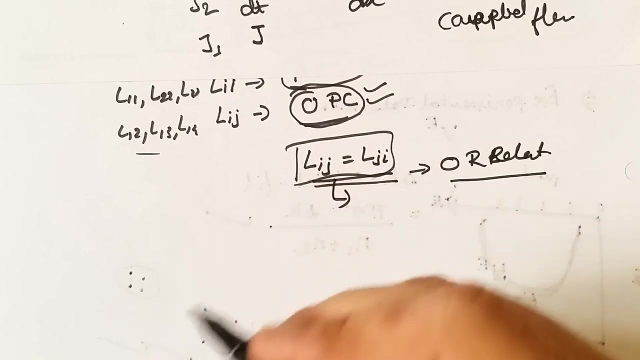 relationship. it is known as Onsager's reciprocal. it is known as Onsager's reciprocal relationship. we will be discussing the detailed derivation in next few lectures to come. okay, and further, further. Onsager: he showed that this relationship exists only for a selected pair of flows, and those flows 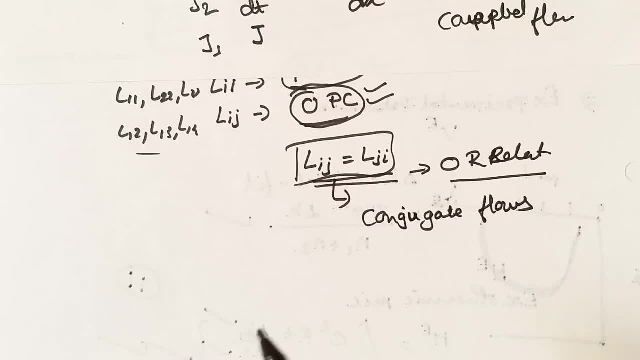 are known as L i j, and this L i j was equal to L j i and this L i j was equal to L j i and this L i j was equal to L j i and this L i j was equal to lost. so this relationship, 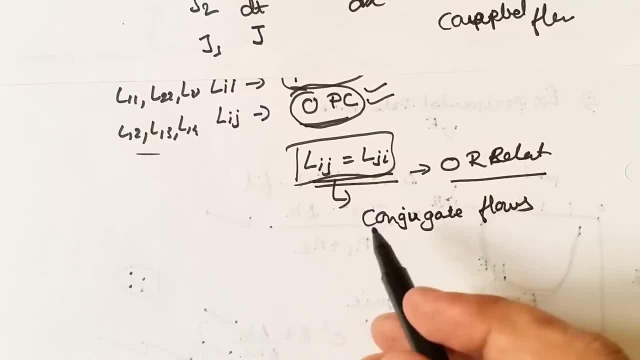 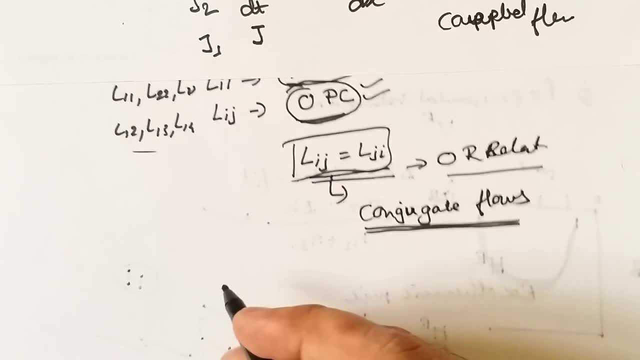 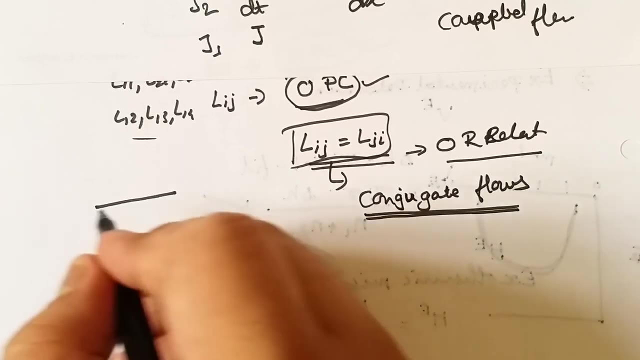 exists only for those flows which helps proper or several selected pairs of flow, and those great flow. so this while known as conjugate flow, so this conjugate flows. let us take one example and understand a conjugate flow. suppose we are considering any one-dimensional conducting. why so in that conducting wire we have? suppose, if we say that via? 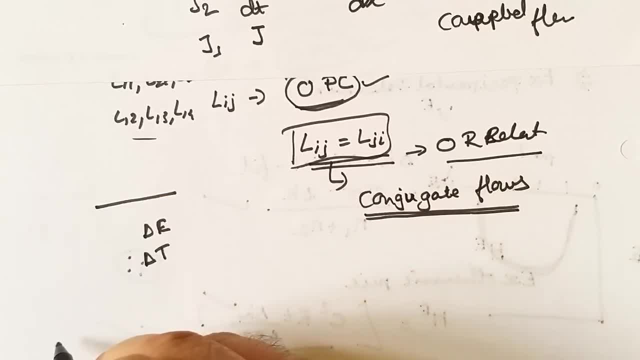 delta is the potential gradient over here, or potential differential gradient, we can difference and Delta T is the temperature difference. then the Delta E and Delta T are the driving force and because of this driving force, because of Delta E, we will. we know that electrical current or J, or we may write as I- is the